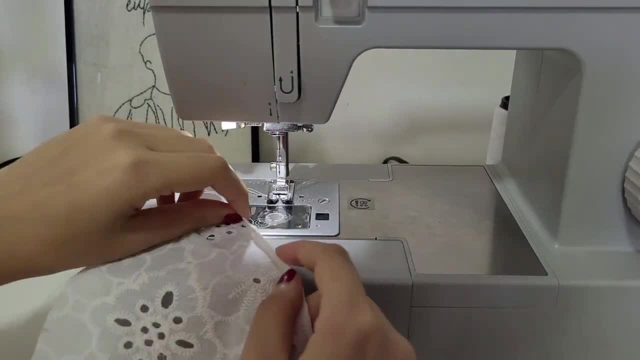 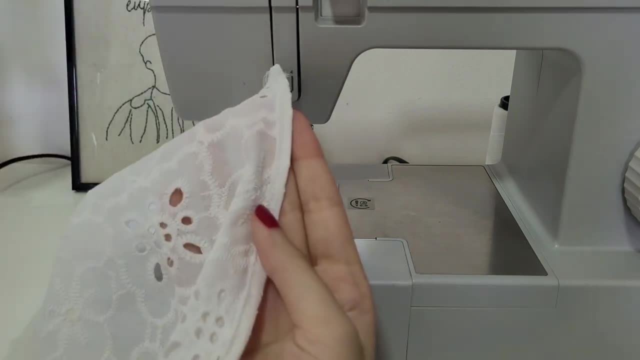 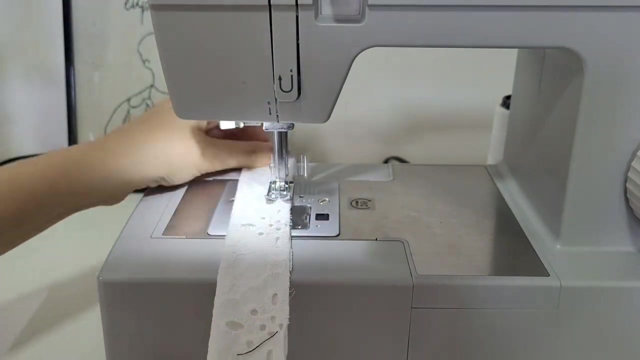 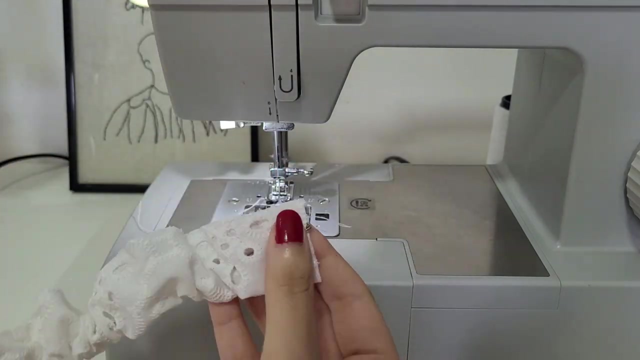 as thin as possible so it looks more delicate. Sew the two pieces together and close it up. I'm using a loop turner for this project, but you can use a safety pin if you like. Now put your elastic inside of it and top-stitch both edges to rural and. 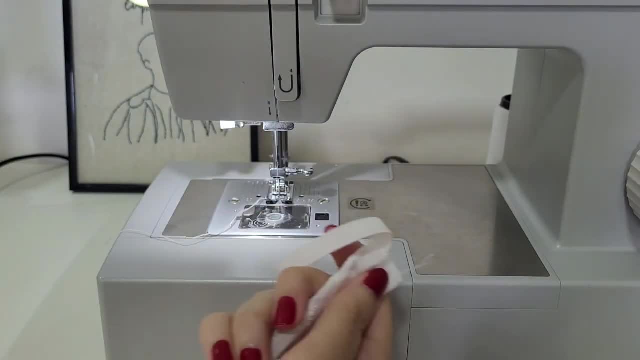 moulth optionally In the refrm section of the video. you should notice I'm screening from the center, So I think I need to tie the shoulder. it enough together to make this a Chansey. That's it. Take our other material and place the other scraps And see you in the next video for. 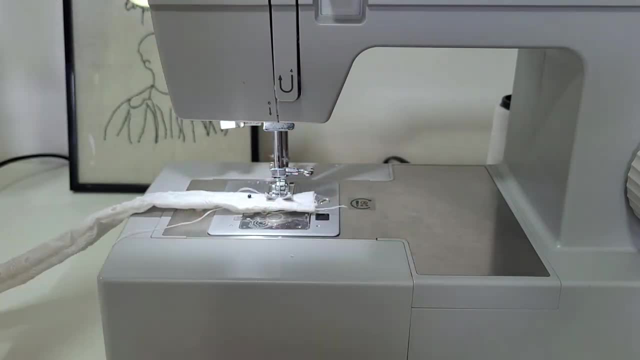 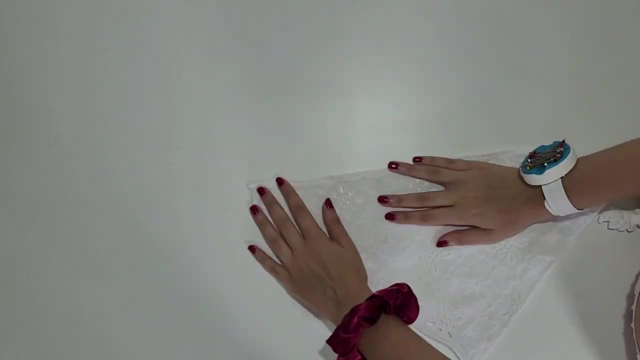 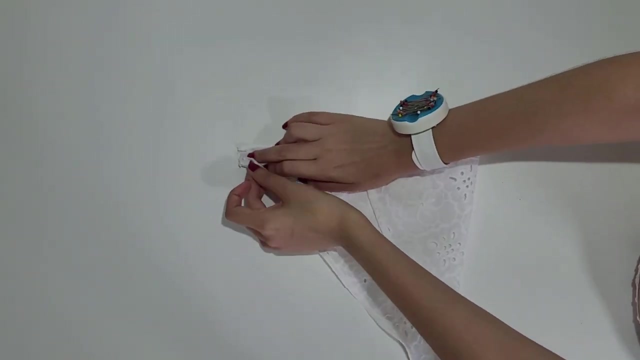 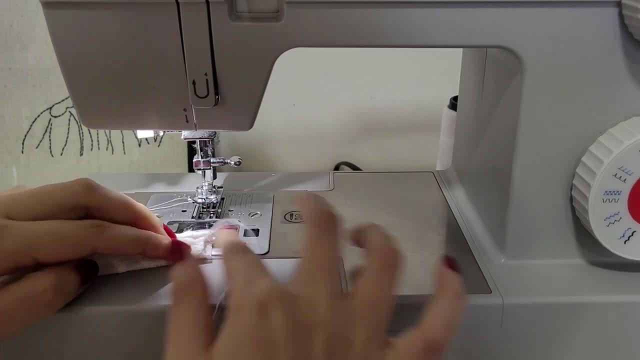 sewing. Um, bye, bye. secure it in place. Now place the band with the elastic at the right side of the fabric that will be facing out and fold the edges on top of it as shown in the video. Then topstitch it in place. 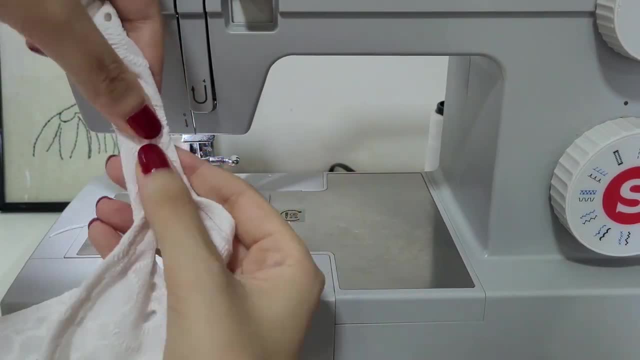 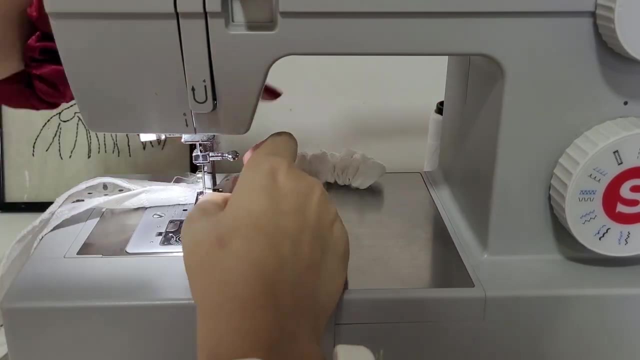 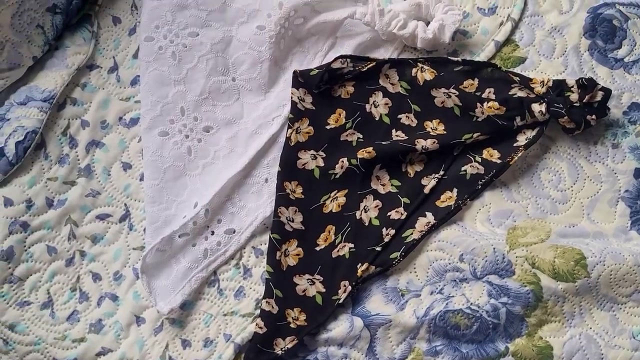 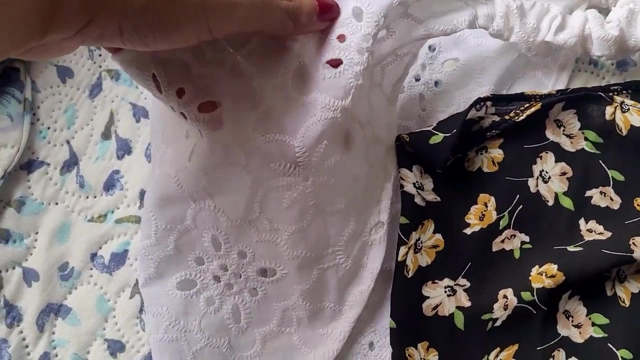 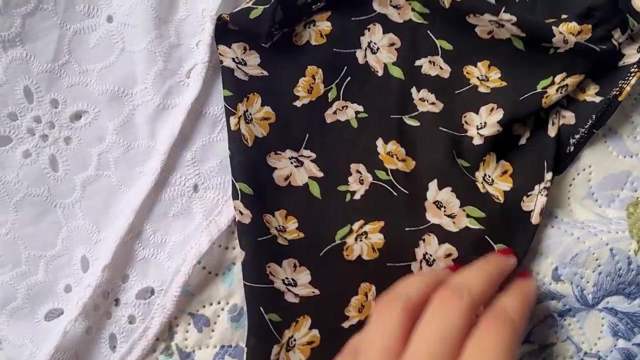 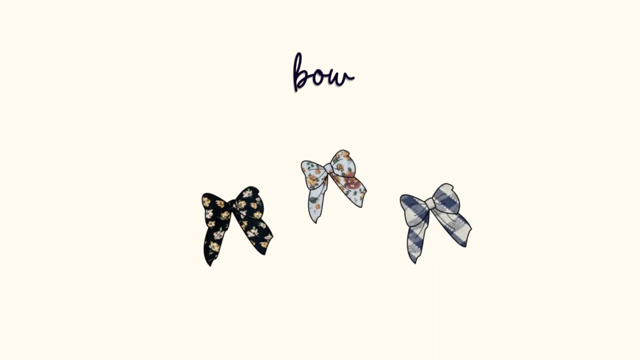 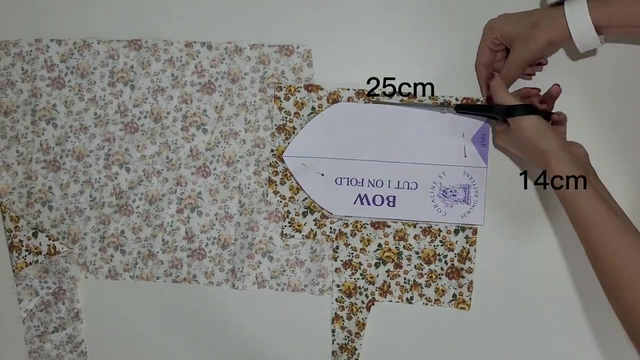 When you turn it inside out, the fold will cover the edge. that's not finished. You can topstitch it there to keep it folded And you're done. Now for the second project. Fold your fabric in half and place the pattern pieces. 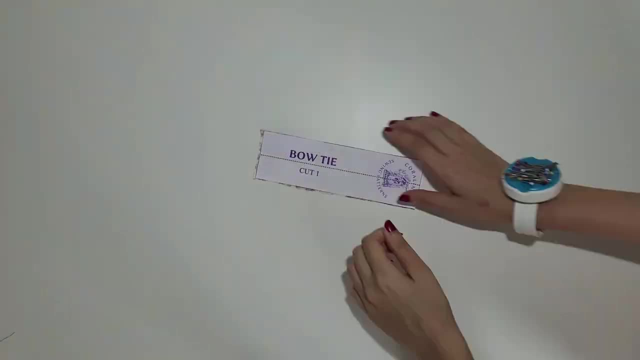 Cut one bow and one tie. Fold the tie in half and stitch it. Then topstitch it in place And you're done. Now for the second project. Fold your fabric in half and place the pattern pieces. You can topstitch it there to keep it folded. 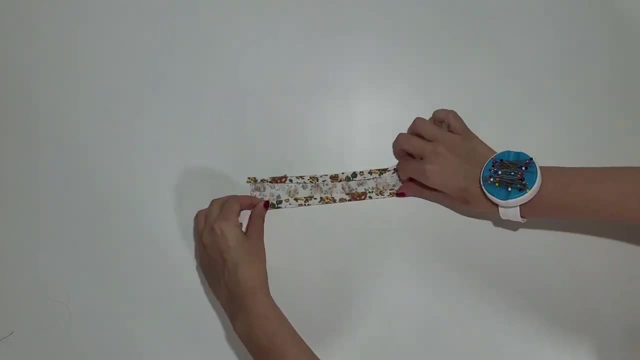 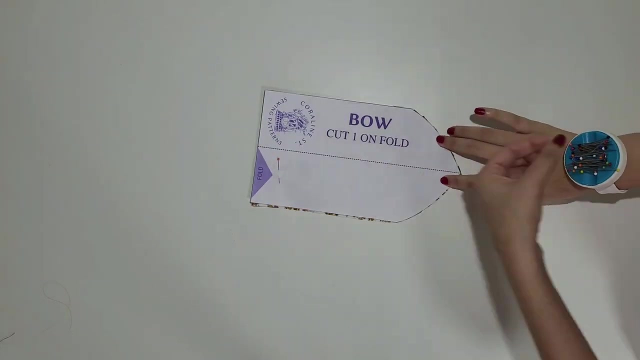 Or fold the edges inside and then in the middle again and stitch it. It's up to you whether you prefer to do it one way or the other. Now for the bow: fold it in half and sew it with a 1cm seam allowance, leaving a space. 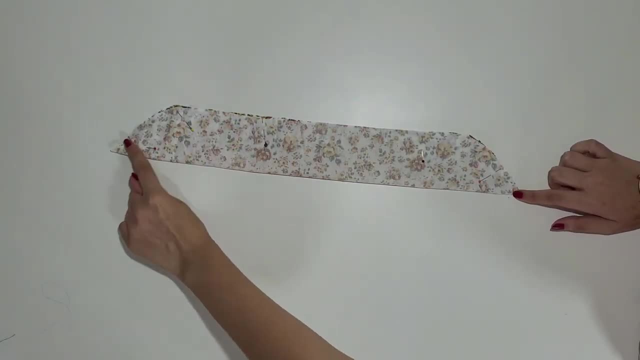 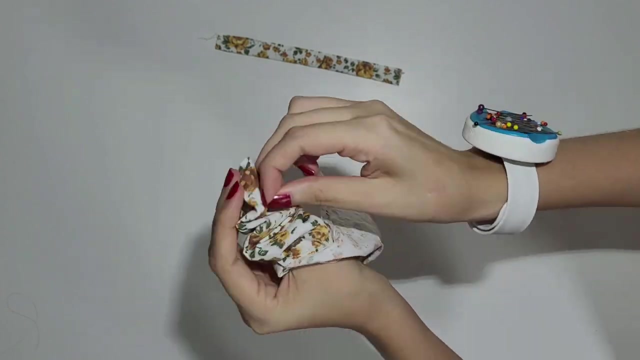 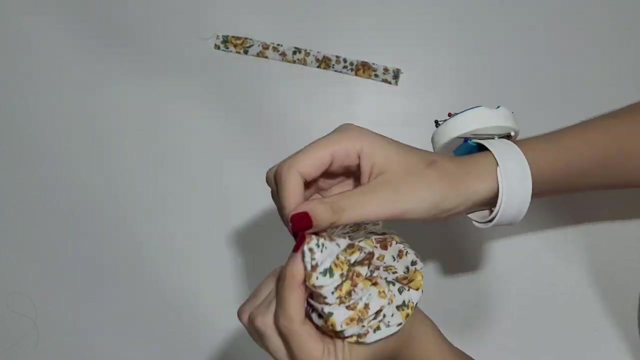 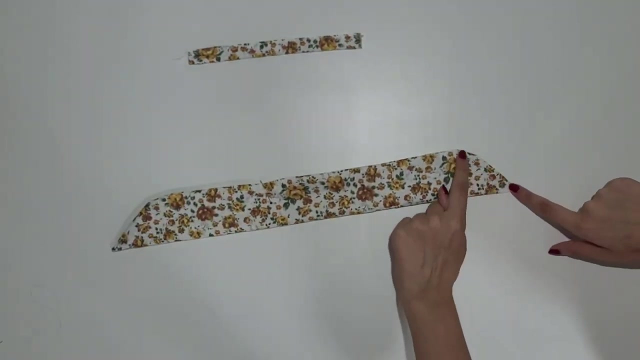 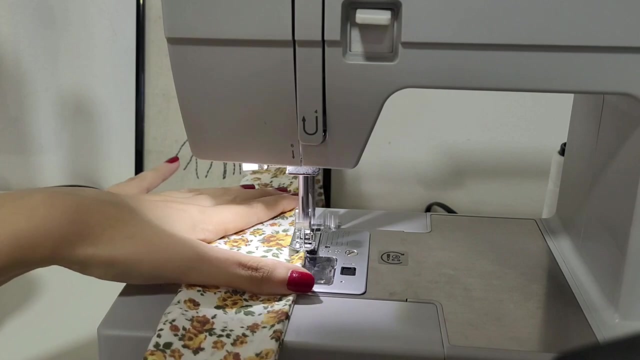 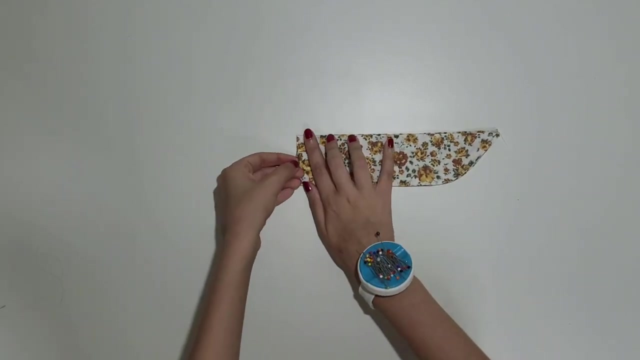 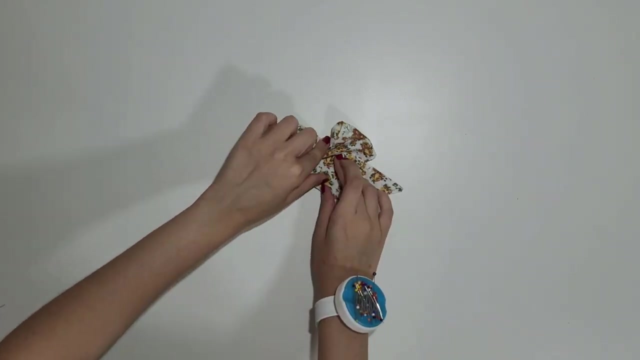 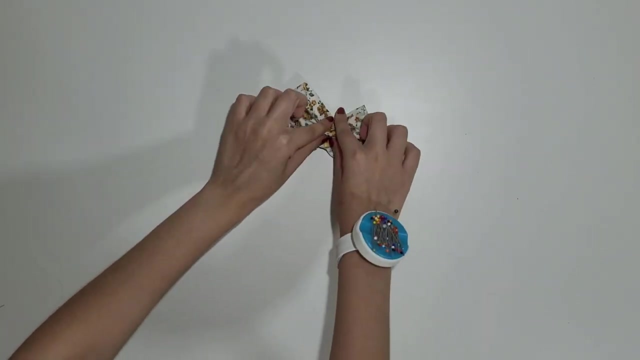 of around 3 fingers without sewing. Now turn it inside out And you're done. Now topstitch it around the entire edge. Now mark the middle And fold both the edges inside, leaving around 4 fingers in the middle. Then pinch the fabric to create the form of the bow. 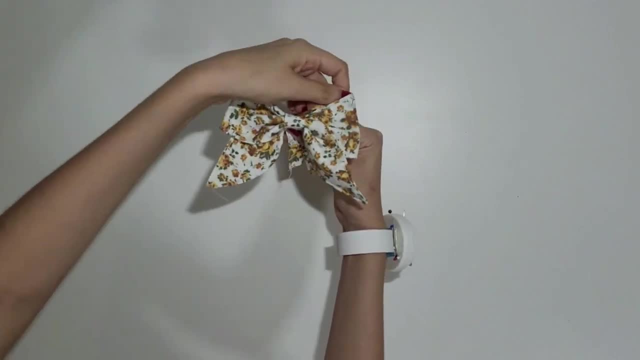 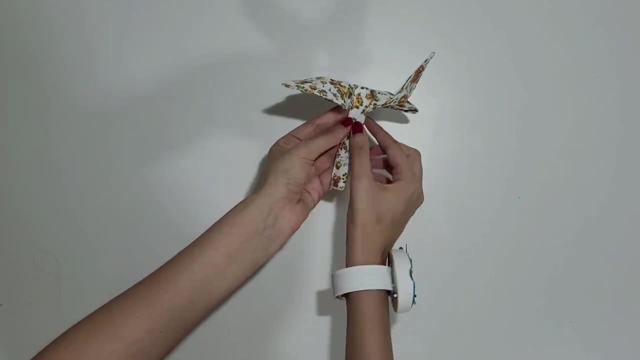 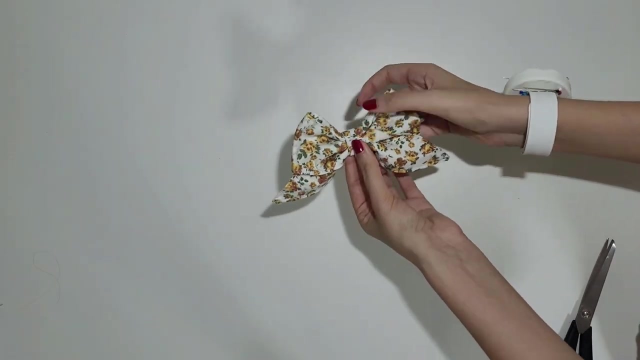 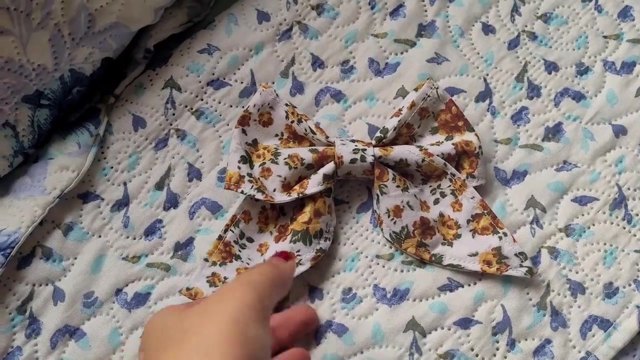 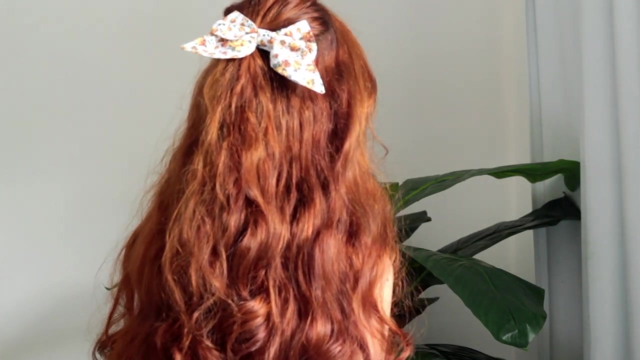 Now use the tie to secure the form and stitch it. You can also use hot glue here if you prefer. You're done. Now you can do whatever you want with your bow. I decided to add a hair pin to use it as a hair accessory. 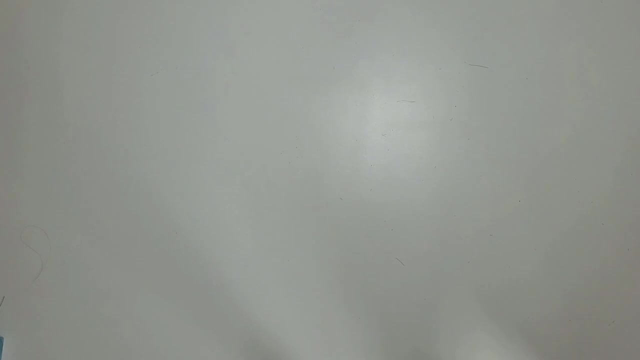 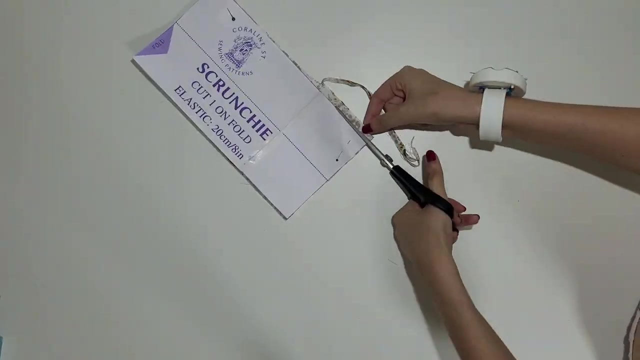 Now for the scrunchie. Fold your fabric in half and stitch it, And you're done. You're done. Now for the dealt-about part. Fold your fabric in half and cut the pattern piece. Fold the edges inside 1cm. 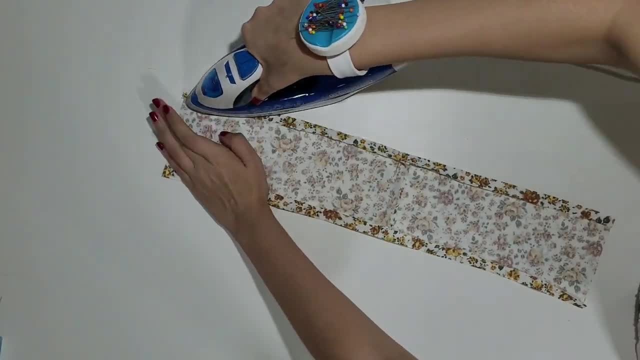 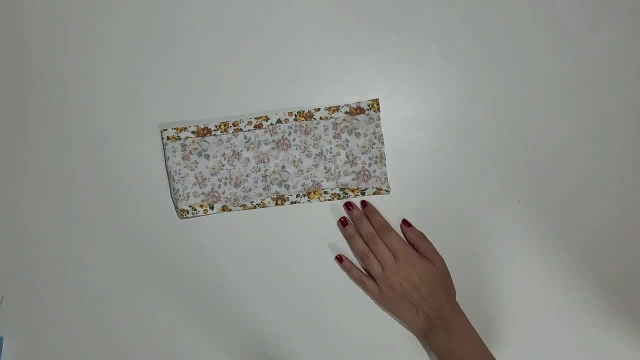 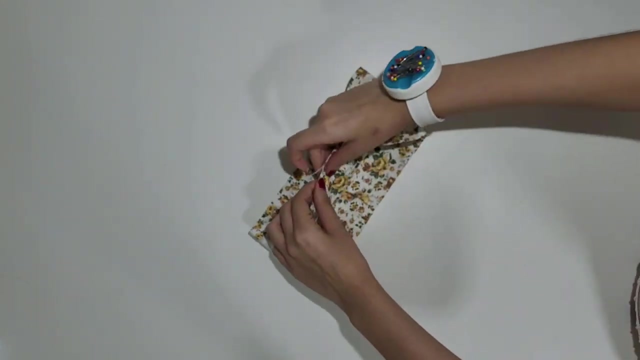 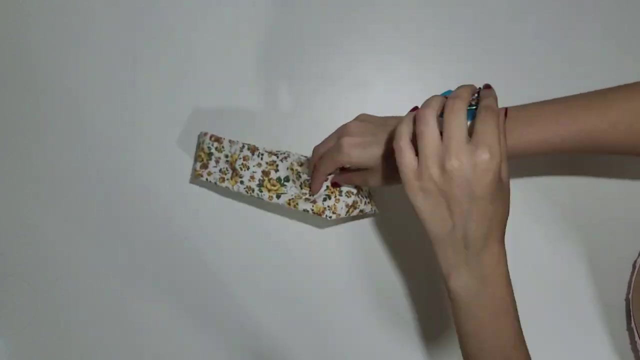 Use the iron to help you. Then sew the edges right sides together After sewing open the seam, and fold the edge in half. Fold the edges to the right, After sewing open the seam, and fold the scrunchie in half. Then topstitch around the edge, leaving a gap to insert the elastic.